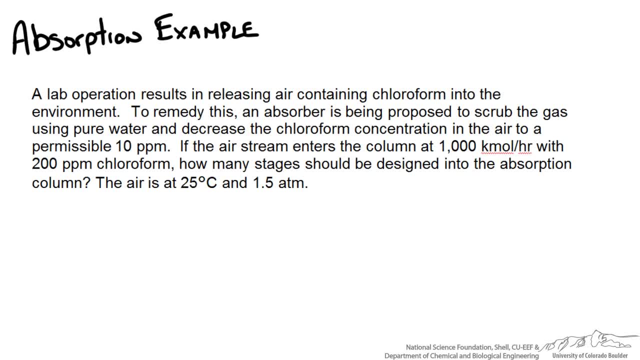 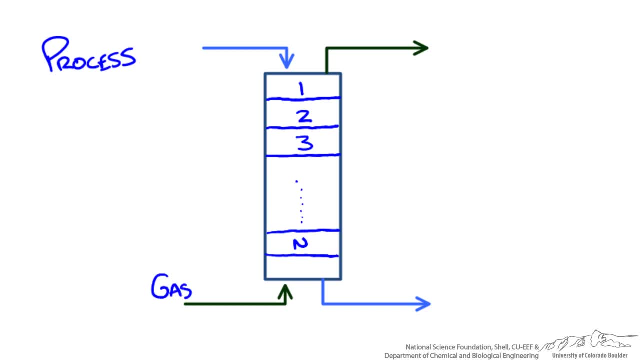 First place to start is with a diagram or a picture of our process. Here I have drawn an absorption column. We have an entering stream here of gas, or, in this case, our air stream containing chloroform. We have gas leaving our column. We are pumping liquid, in this case water, to the top of our column so that it flows. 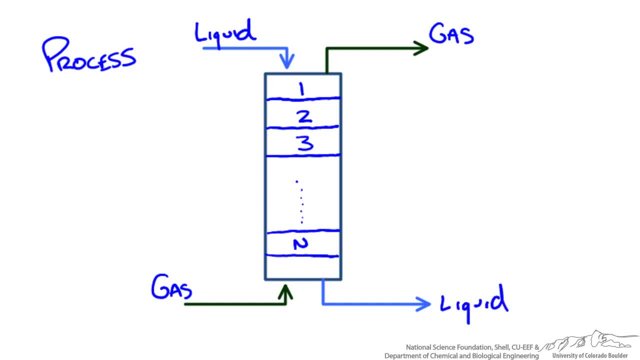 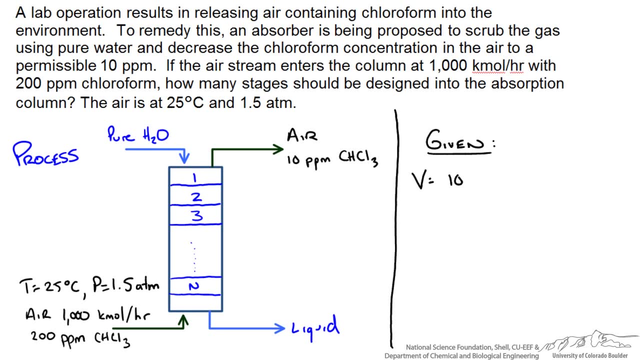 downwards and we get our liquid leaving the column. Let me fill in some details that we know. So we are given a vapor flow rate of 1000 kmol an hour. We are given an inlet concentration of 200 ppm, which is a mole ratio, but since we are working with really dilute solutions, 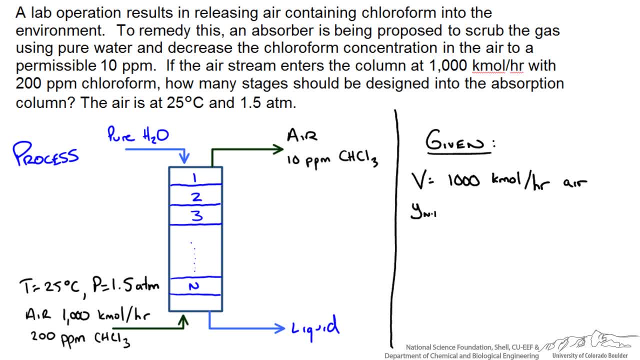 we could write it as a mole fraction. So our fraction of chloroform entering is 200 parts per million. So for every million parts of air we have 200 parts of our chloroform. We are also told the concentration leaving needs to be 10 parts per million. Since we are using pure water, we know the concentration coming. 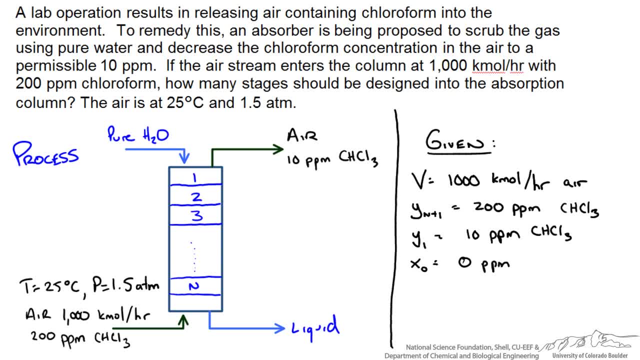 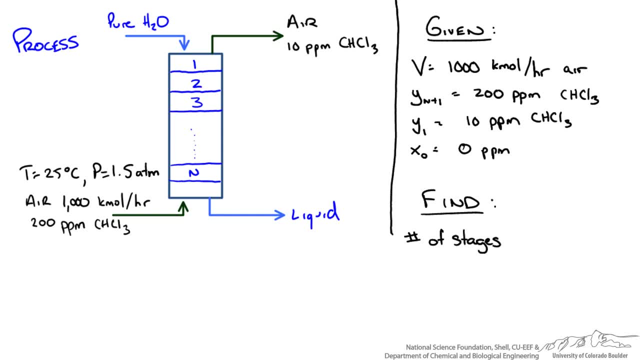 in of chloroform in the water stream is 0, and that is all we are given. We are asked to determine the number of stages for this column. The question now becomes: is this something we can solve? We can use a degree of freedom analysis For a single section: countercurrent. 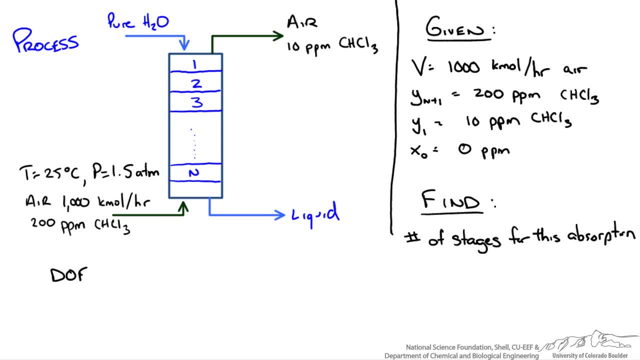 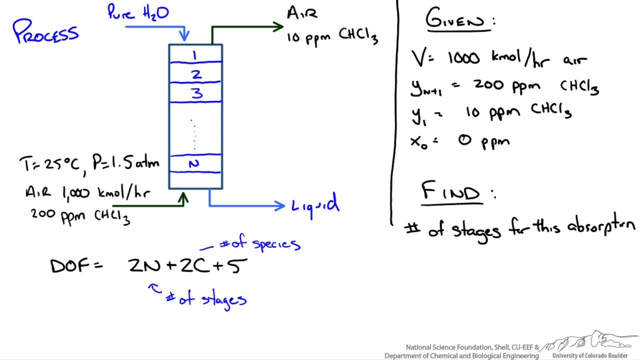 cascade, our degrees of freedom will be equivalent to the following: Where n is our number of stages, c is our number of species. So at this point we need to make some assumption so that we can a, a minimize the amount of variables that we may need to find or look up. If we say that each 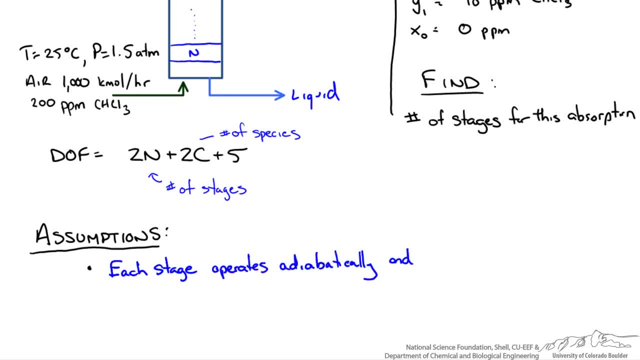 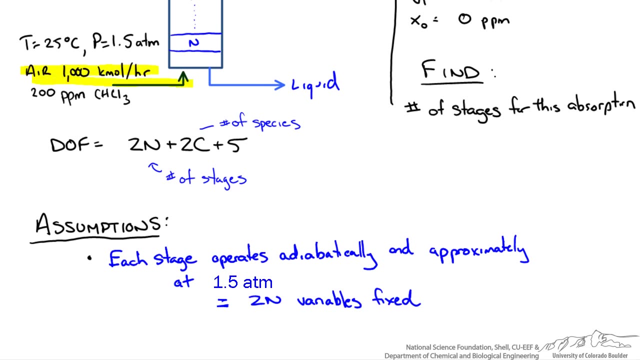 stage operates adiabatically and there is no pressure drop along the column, then we will fix the amount of variables equivalent to the amount of stages times 2.. Looking at our incoming stream, here it is completely specified: temperature, pressure, composition and flow rate. therefore, taking C plus 2 variables up. Now for our liquid feed, we are told that 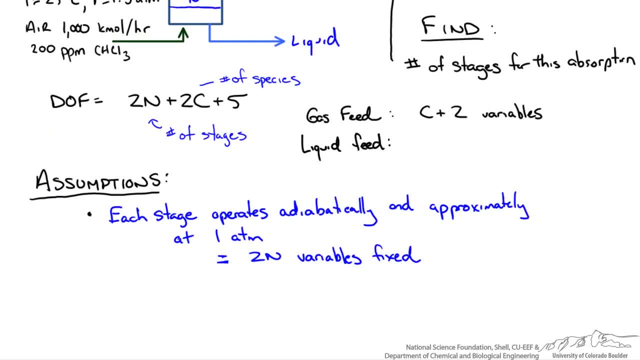 it is pure water, but that is about it. So we could assume that the entering liquid is also at 25 degrees. but we are not given a flow rate for the liquid, so we only fix C plus 1 variables If we take into consideration how many we could fix with our assumption. 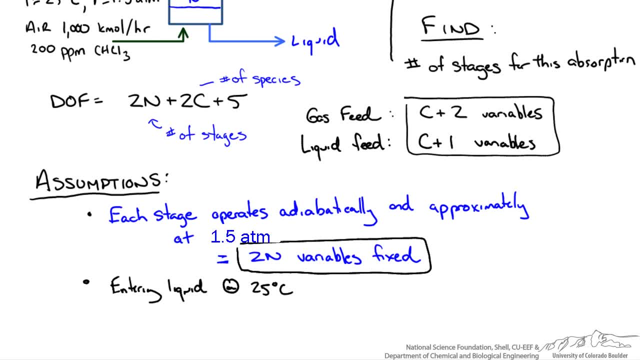 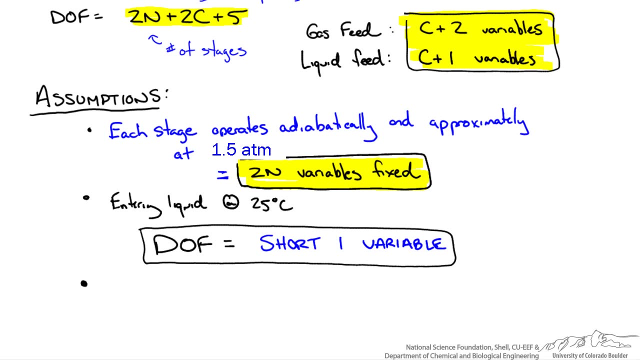 and how many we are given. We can compare this to our degrees of freedom from our absorption column and you can see that we are short. one variable, As mentioned, this is going to be the flow rate of our stream. So we need to make another assumption. The flow rate for an absorbent can be related. 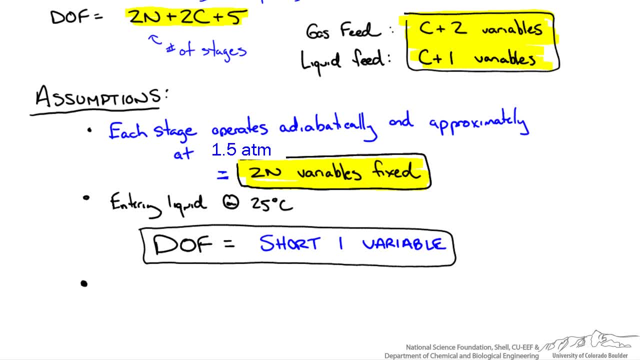 to L over V min. So good operating condition for our absorbent flow rate is typically somewhere in the ballpark of 1.4 times the minimum absorbency flow rate. So we are going to assume that our flow rate L is going to be 1.4 L min. 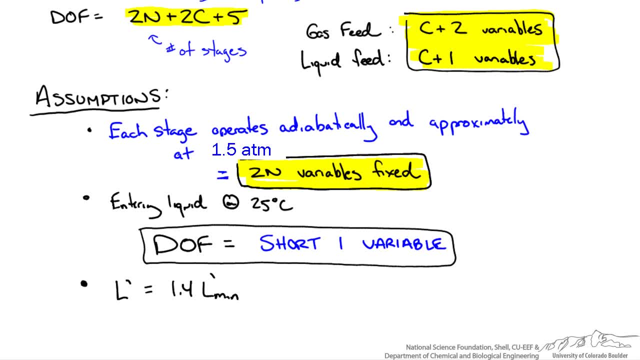 So we need to figure out what that minimum flow rate would be for our system. Typically, a good ballpark range here is between 1.1 and 2 times that minimum flow rate. Now we have specified L prime and we can find L min. One more major assumption we need to make: 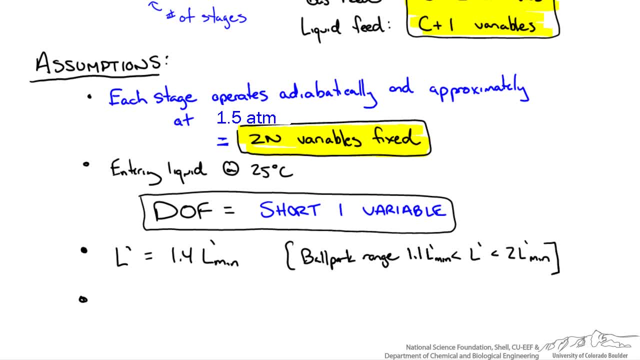 in this case is that, since we are working with very low concentrations of chloroform, that we are going to assume that no water is stripped into the gas stream and no air is condensed into our liquid stream. That being said, our flow rates for our liquid and 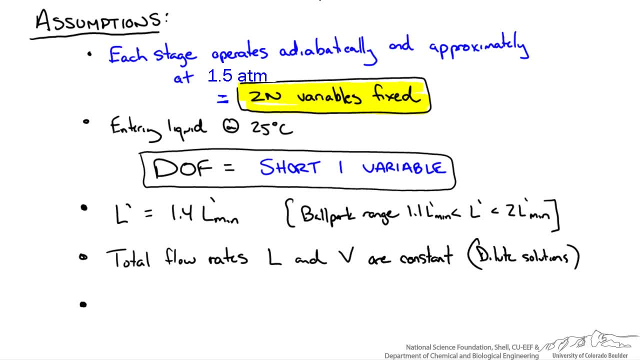 vapor will be constant. And lastly, because we are working with very dilute solutions. typically for an absorption problem, we would be using Y or big X to signify mole ratios, But these can be appropriate for any type of dilute solution. So what we are going to 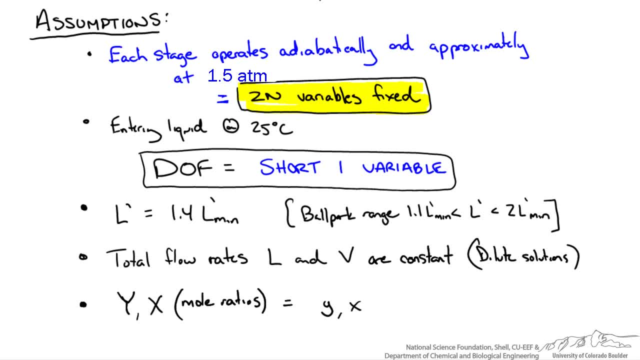 do is approximate by the mole fractions, since we are at very low concentrations In this case. as our mole fractions approach zero, our mole ratios approach our values for the mole fractions. So we can plot for the McCabe-Thiele diagram just in terms of the parts per million. 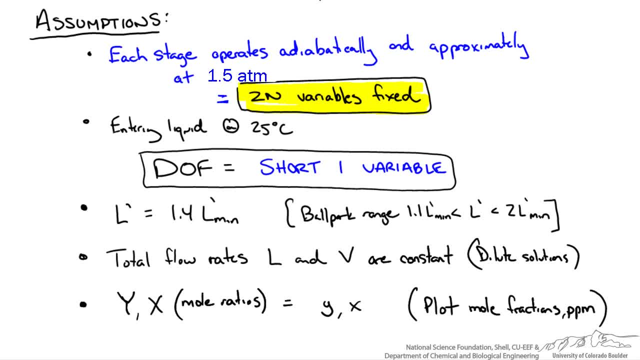 as our mole fractions. And lastly, the only thing we need left, not an assumption, but is to pick some kind of phase equilibrium information for this system And in this case, with chloroform at the concentrations we are using, we can assume Henry's law, Which we 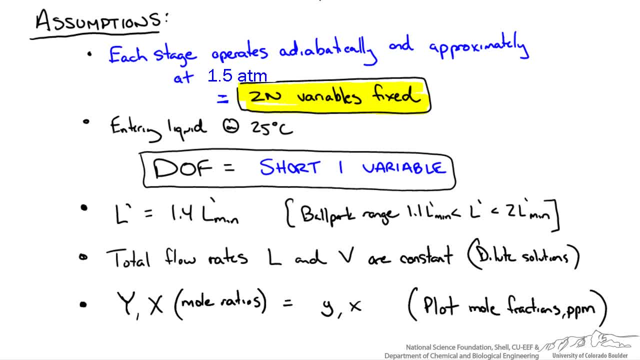 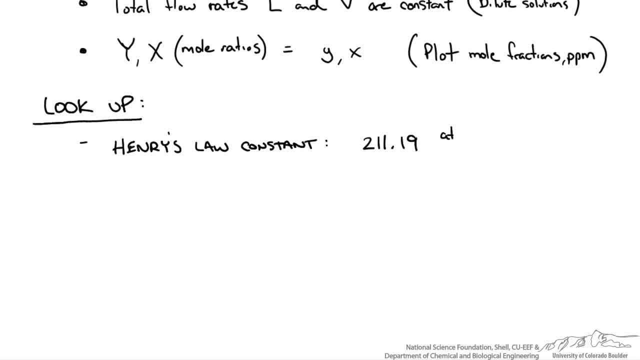 can look up for the system in a handbook and see that chloroform has a Henry's law constant of 211.19 and this is atmosphere per mole fraction in water: 25 degrees Celsius and 1 atmosphere. So using Henry's law we could figure out what our phase equilibrium line is going to look like In this problem we have. 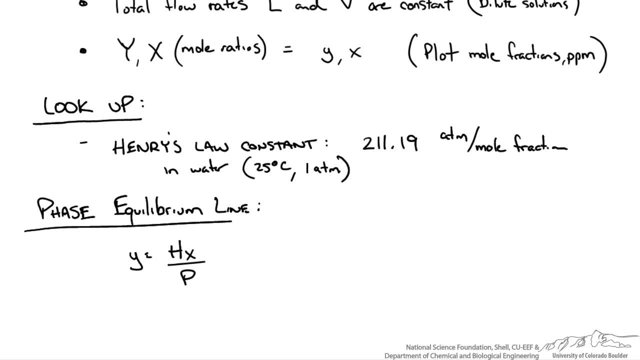 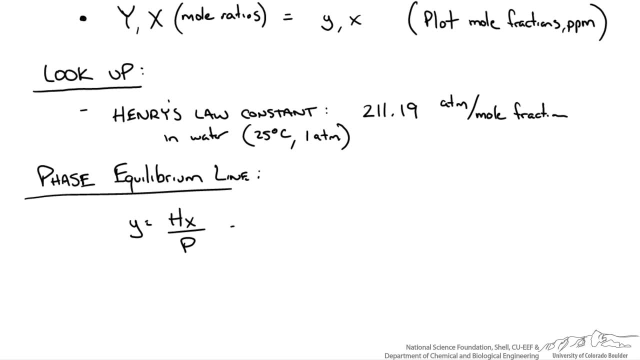 We could figure out what our phase equilibrium line is going to look like In this problem we have. In this problem we have looked up Henry's constant and we know the pressure that our absorber is going to operate at. so we could get a relationship between y and x. So you can see, this is a straight. 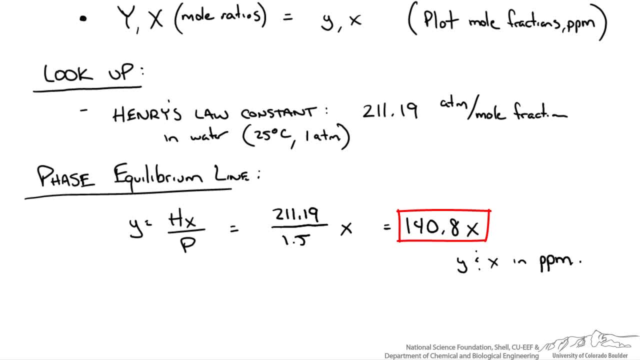 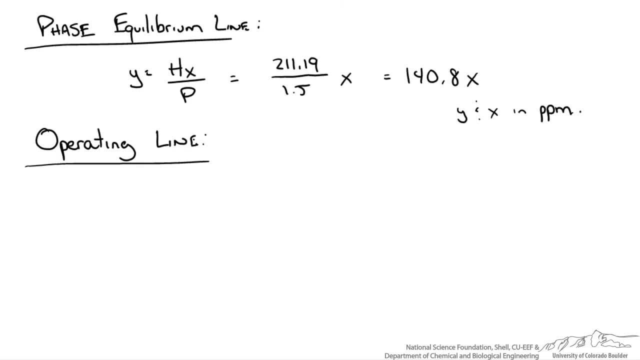 line with a slope of 140.8 that goes through the origin. So we could plot this on a y versus x plot along with our operating lines. So for our operating line we want to work in the appropriate region of our concentrations So to determine the extent at which our phase 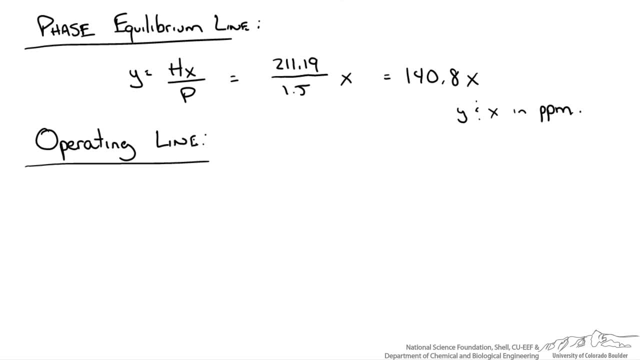 equilibrium line extends. we could take the concentration that we start with, the 200 parts per million, and divide it by our phase equilibrium slope. The concentration in the liquid phase will be at equilibrium Based on our column. we know exactly what one of the points on 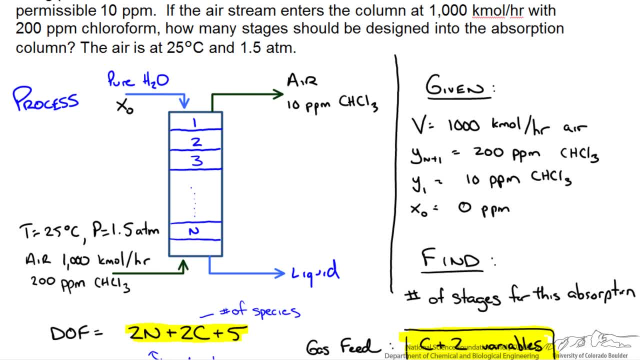 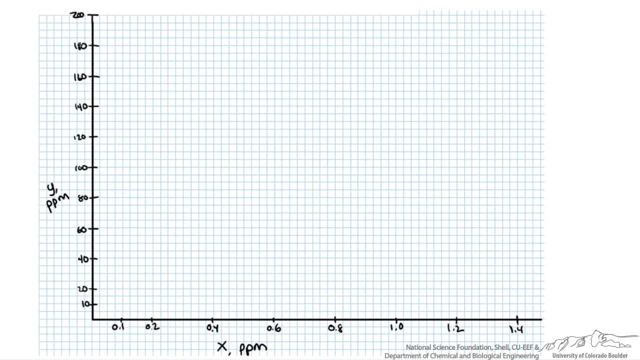 our operating line will be: We have x0 equals 0 and we have y1 is equal to 10 parts per million. So the top of our column or the bottom of our operating line will go through the point. So here we have a plot that we can start working with. Obviously, you can see that the y and x axes 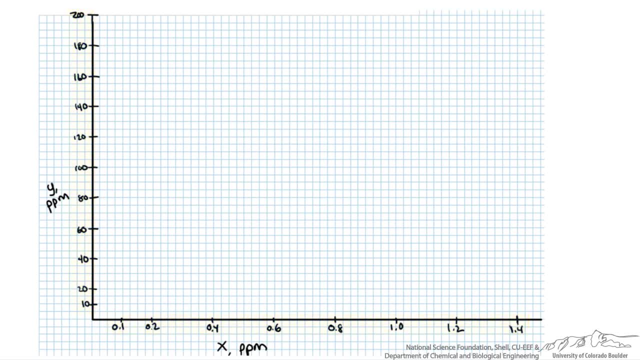 are not equal. We do know that the equilibrium line at 200 parts per million for y will be 1.42 for x. So that puts us right about here, and we know that it goes through the origin. So this is our phase equilibrium line. We also know that the bottom of our operating condition is going. 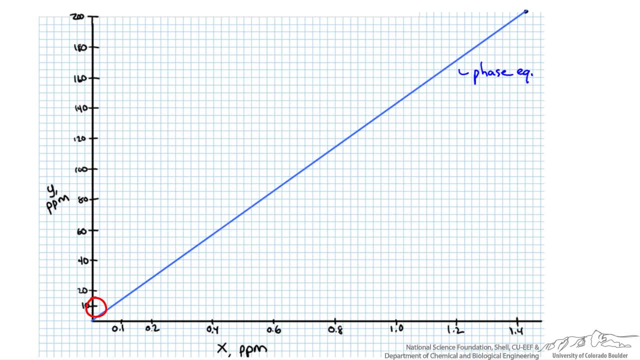 to be 0 for x and 10.. So if we wanted to determine at this point what the minimum absorbent flow rate would be, We are looking for Lmin. That is going to correlate with an infinite amount of stages. So this is what our operating condition is going to be. This is what our operating condition is going to be. 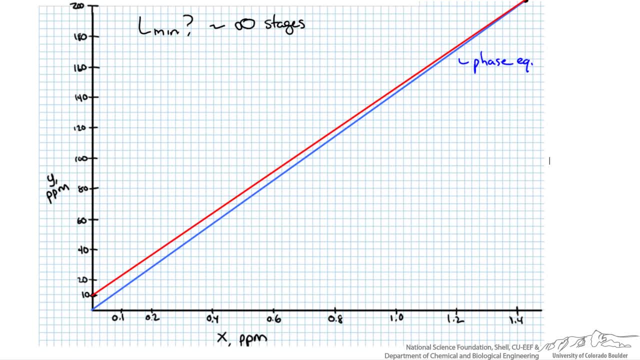 This is what our operating line would look like if we had an infinite amount of stages counted off between our operating line and our phase equilibrium line. As you see, that gap becomes smaller and smaller. So we could determine what the slope of this line would be, because that will give us an idea of what our L and V ratio is, and then we can multiply. 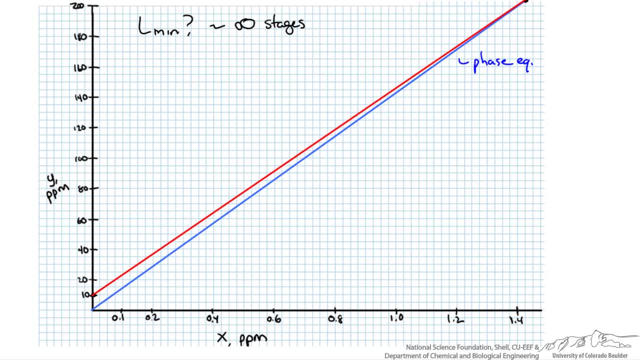 that by our factor 1.4 to draw our actual operating line. So in this case we have 200 minus 10 for our change in y And we have 1.42.. We have 1.42 minus 0 for our change in x, We get a slope of 133.8.. If you recall our 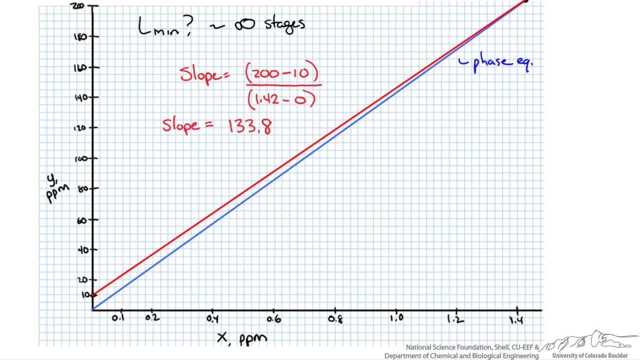 operating line for an absorber is y equals our ratio of our liquid to vapor flow rate times our composition liquid phase plus our other conditions both leaving and entering our column. So the slope of this line is L over V. So we have now determined L over V. 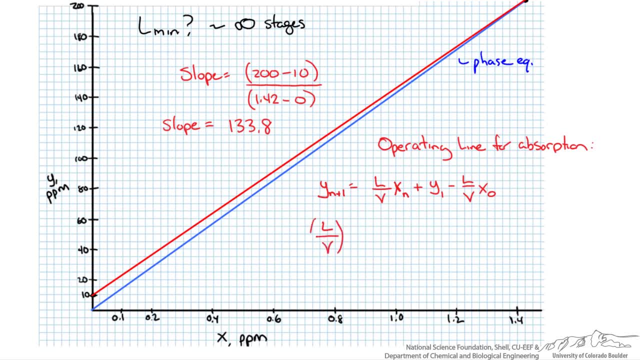 minimum as 133.8.. And we want to operate at 1.4 times L min and that gives us 187.3.. And we could plot a new operating line through the same initial point 0, 10, with a new slope. 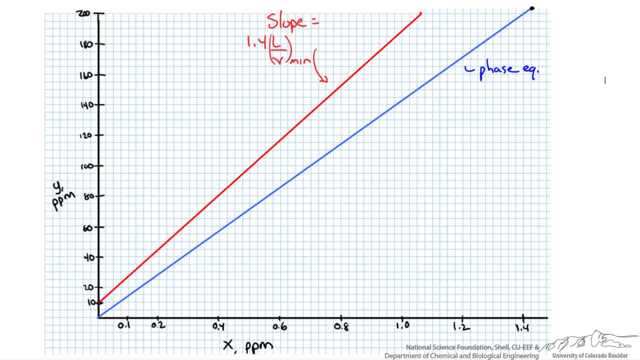 of 187.3.. So using our ratio 1.4 to the L over V min, we could plot our actual operating line for our system. We could solve for x And in this case and see that it is about 1.06.. 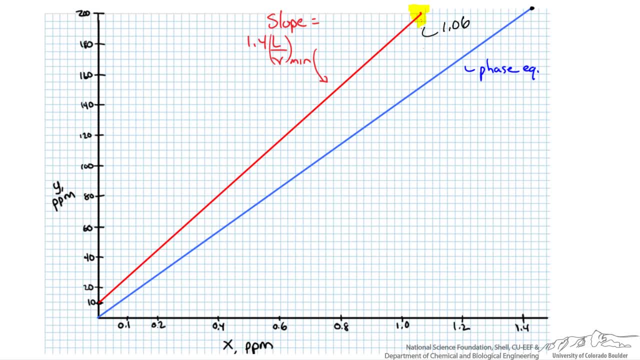 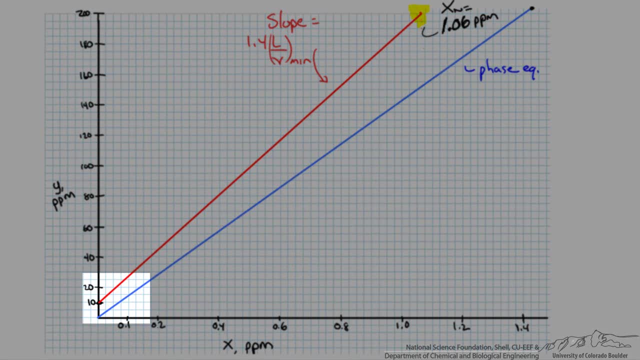 So now that we know our outlet condition, we have our operating line, our phase equilibrium line, we could start counting our stages. So we start at the conditions for the top down. here We go exactly horizontal over to our phase equilibrium line. We go straight up to our operating line.